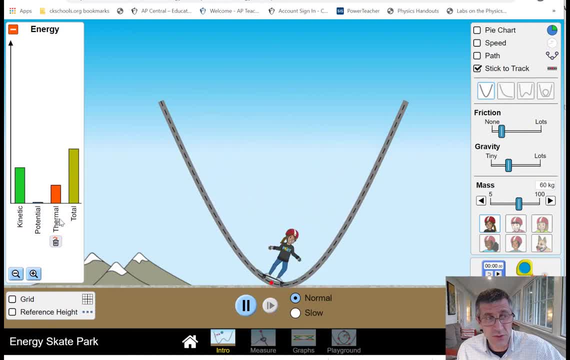 losing that energy into thermal, so it's becoming less useful. So my total energy is conserved, But my kinetic and potential energy, or I'll call my mechanical energy, is not conserving. my kinetic energy, Energy is not being conserved, and so I'm losing some of it. 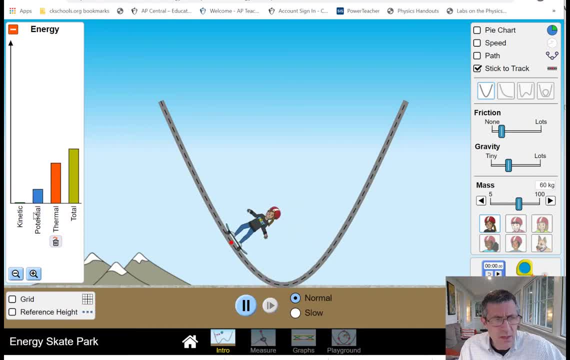 So I'm going to be careful about how I describe some things. So energy: we'll have conservation of energy and we can pretty much only lose it through friction in this friction and drag. So there are a couple of handy ways of thinking about this. 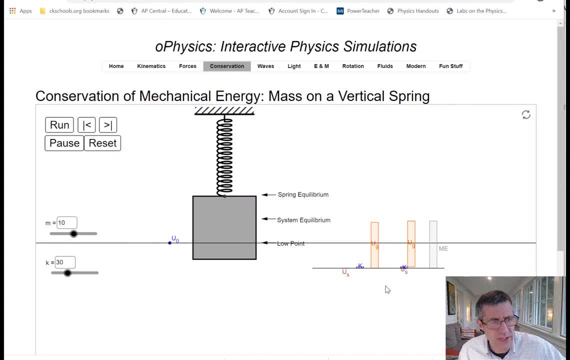 So here's another example, And again I like these bar charts on the side as a way to describe this. So what I'm going to do, I'm going to start this thing in oscillation- oscillation, so it's going to be moving up and down. 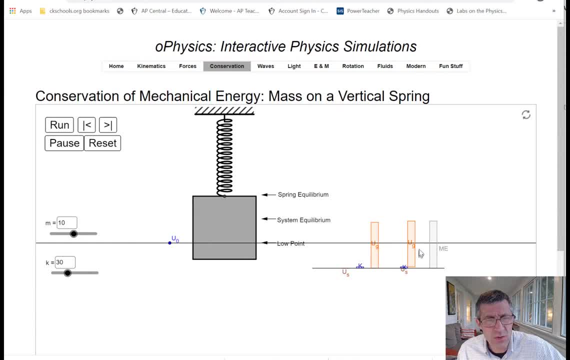 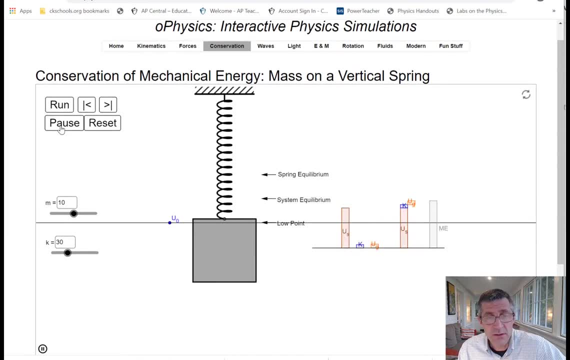 Notice, my total mechanical energy is going to stay constant. So right now this is all gravitational potential energy And as I run it that's going to shift. Now I've got some spring energy and a little bit kinetic, and then spring gravitation. 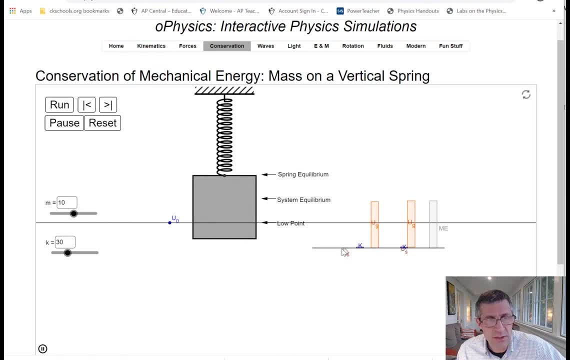 Now, if I look at these three separately, right, so my spring energy, as my spring gets stretched, I'm storing more energy there. As it goes higher, as my moccasin goes higher, I'm storing more gravitational. But notice, these three add together to equal mechanical energy. 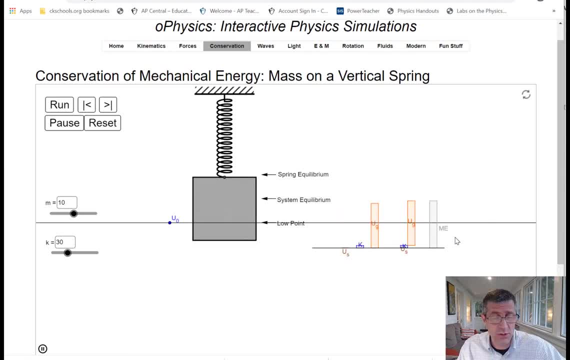 So I'm not losing any energy in this. There's no friction that I'm worried about, no drag, no torsional loss in the spring that I've got mechanical energy which is conserved. So these bar charts are a really handy way of thinking about it. 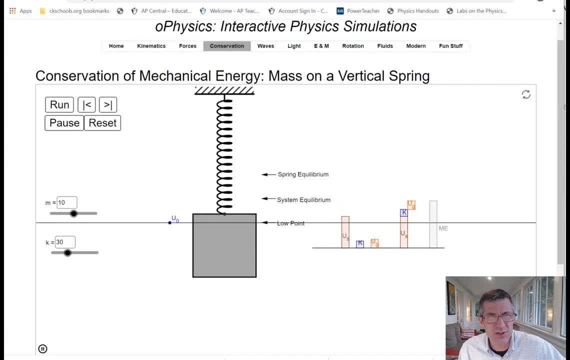 But notice, there's got to be something to start this in motion, right? So just like with my skateboarder. oh, I agree, she's got to stop right, My skateboarder. I had to get her someplace right. 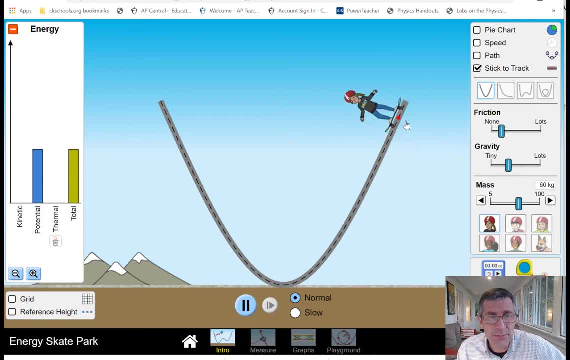 So how did I start this all? Well, I lifted the skateboarder up to the top right, So I did some work. I applied some force against gravity along some distance, So I applied some force over some distance to get here to the top. 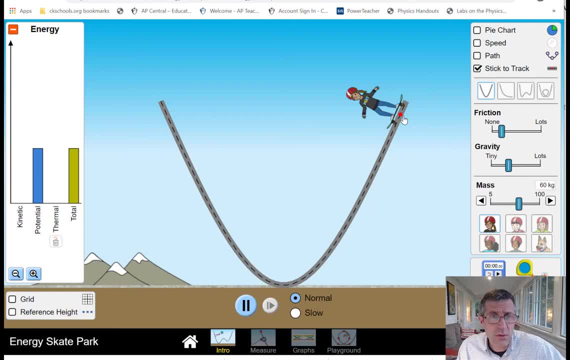 So now I put energy into my system. So work is the only way that we have in this class of adding energy into a system And technically it's the only way that we'll have it take an energy out of the system. So I'm going to think of friction as being some frictional force over some distance. 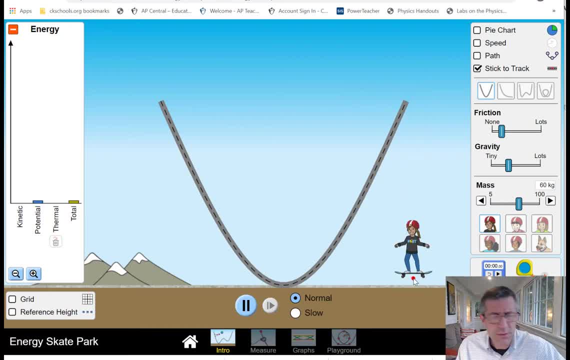 that's acting to remove energy from the system. So let me describe a way that we'll think about this. So let me go back to- yeah, I guess to the skateboarder And let's draw something out so we can see how it's going to look. 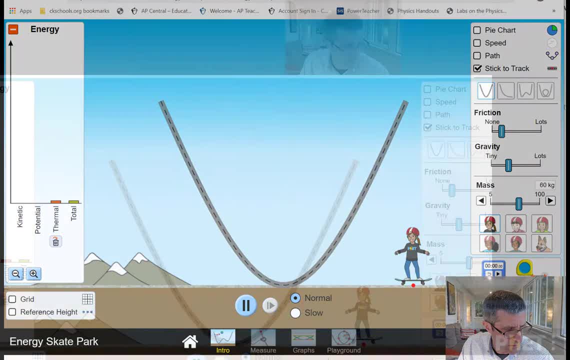 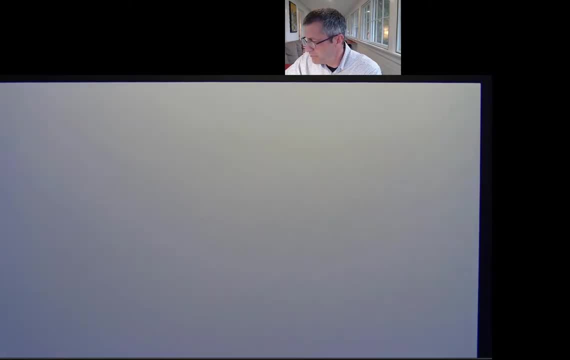 And the way that we use these systems is really handy. So let's see where this goes Here. it is right, So this is how I'm going to. I want to think about these, So I'm going to have a before and after. 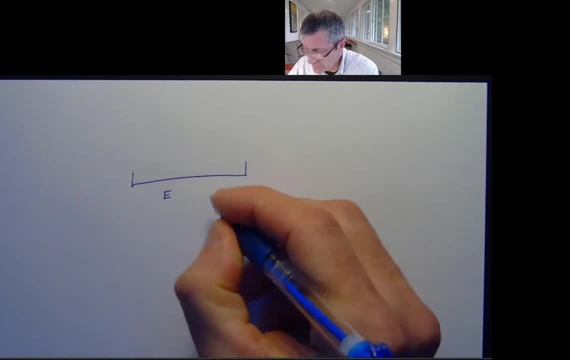 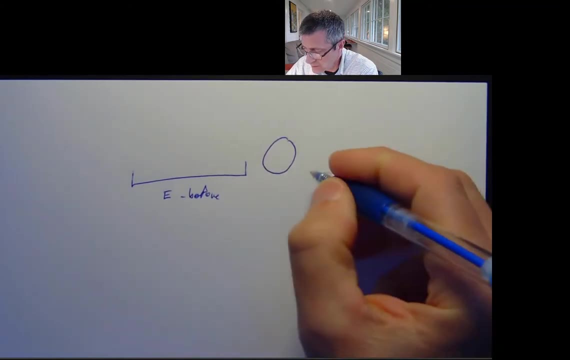 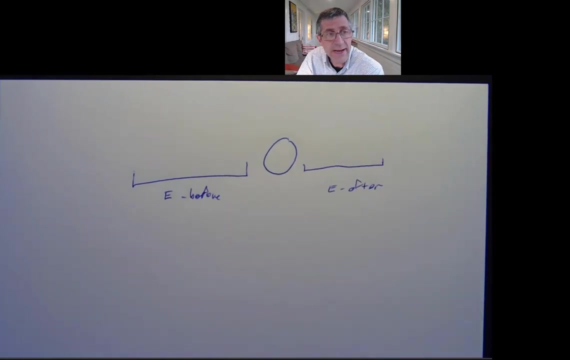 I'm going to say, well, here's my energy that I have before I can do something to my system, And then I'm going to have some energy afterwards. So, for instance, if I have this spring, that's moving back and forth. 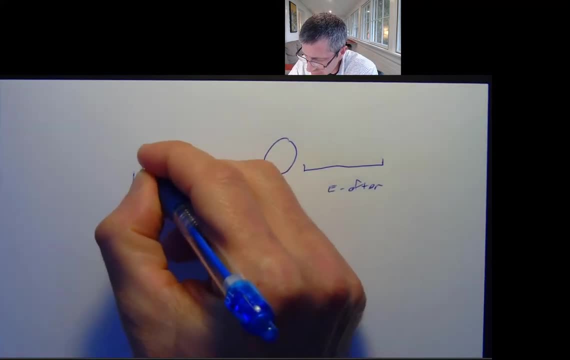 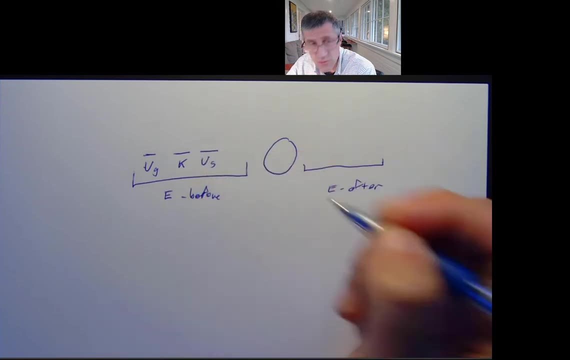 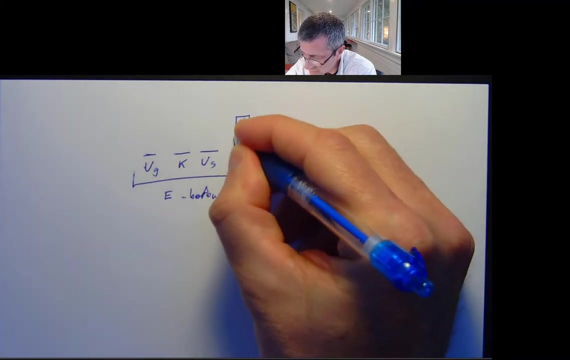 I may start here with gravitational potential energy And that may move to kinetic energy And that may move to potential spring energy And my total energy right. This is always going to be the same right. My total energy before and my total energy afterwards is going to be the same. 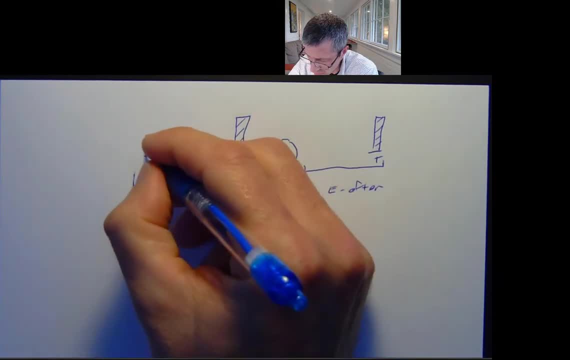 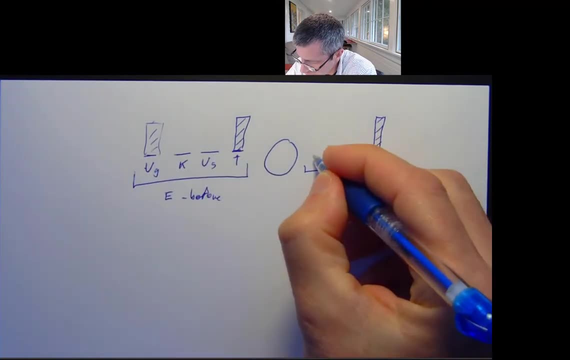 Imagine those are the same height And what happens? right? So maybe I start with a lot of gravitational potential energy. I start with all gravitational potential energy. I'm going to map to my top. When I get to the bottom I'm going to have gravitational potential kinetic spring energy. 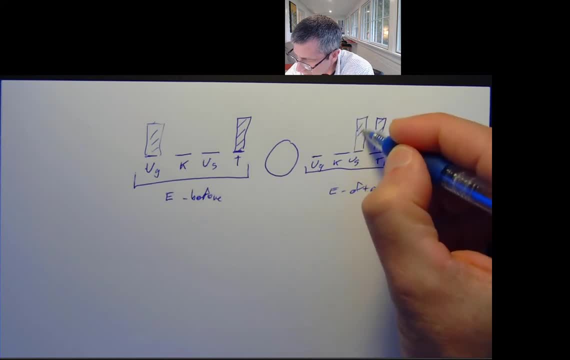 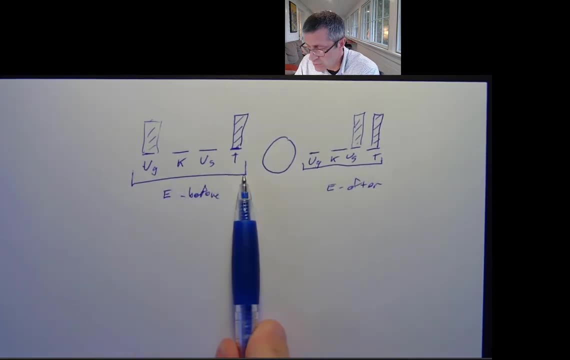 When I get to the bottom, I'm going to have all spring energy, And so this is one way that we like to represent this. So notice, Notice what I'm saying. I'm saying that here I started with gravitational potential energy and this much total energy. 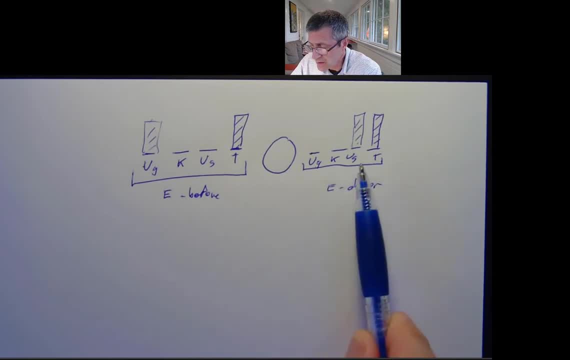 And then when I got to the bottom right- So the second thing I'm interested in, it was all in my spring- I had the same amount of total energy. So there are circumstances where I may be adding work into something. So if I start, for instance, with a car that's at rest, 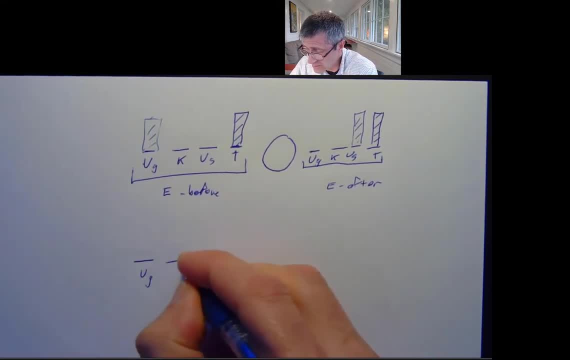 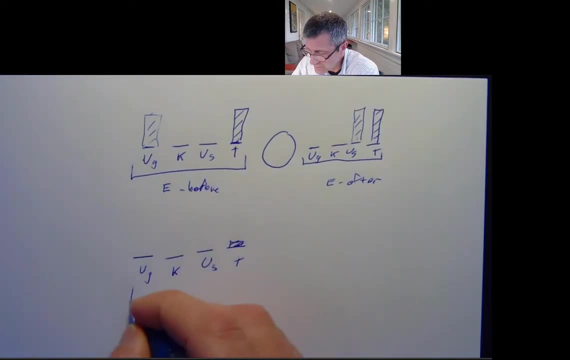 So if a car is at rest, I have no gravitational potential energy, no kinetic energy, no spring energy, No energy, No energy. Total energy is going to be zero. So this is what I had before. This is the energy before. 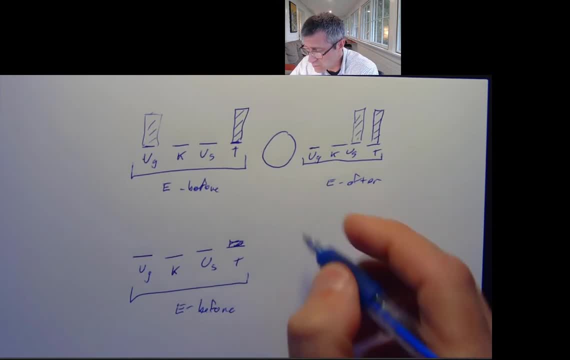 If I push that car, I'm doing work. So what am I doing? Well, I'm taking my system and I'm adding energy into it. So I'm doing work And I'm going to end up having at the end of that- well, maybe I just have kinetic energy now. 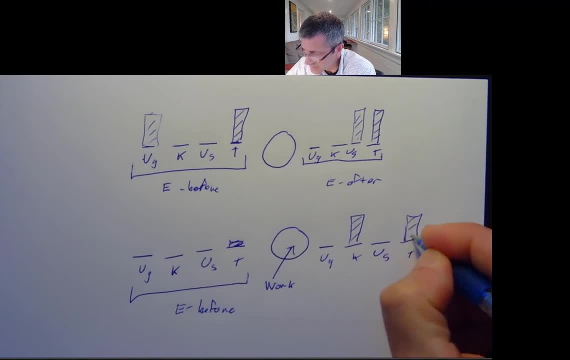 No spring And my total energy now is going to be higher, Right? So notice: In this case, this is not energy conservation, right So? this is not mechanical energy that had beforehand being conserved and afterwards, right So my mechanical energy was less at the beginning, but I added energy in through work. 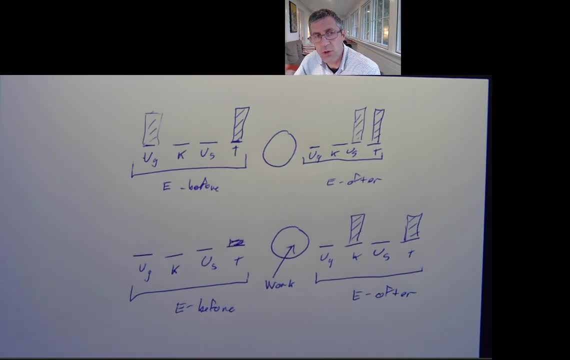 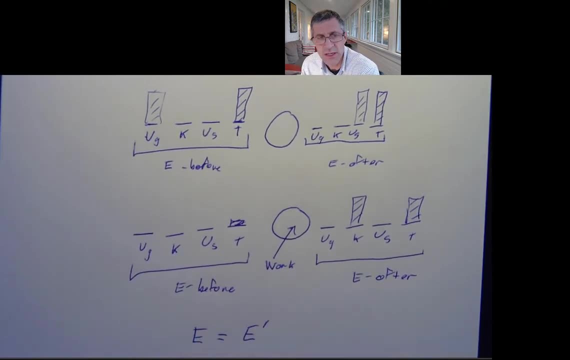 And now I have more mechanical energy. So we're going to have ways of getting to equations, And what I want to do is always start with the same idea. So the energy before is going to be equal to the energy afterwards, And I'm going to take work into account. 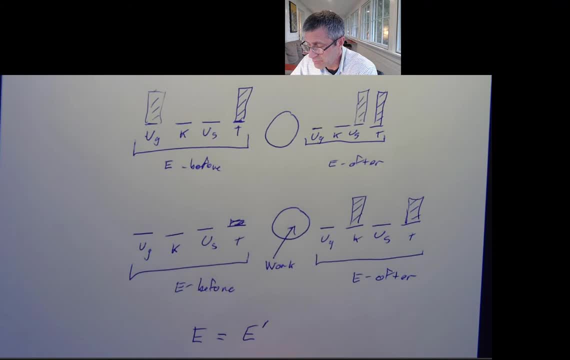 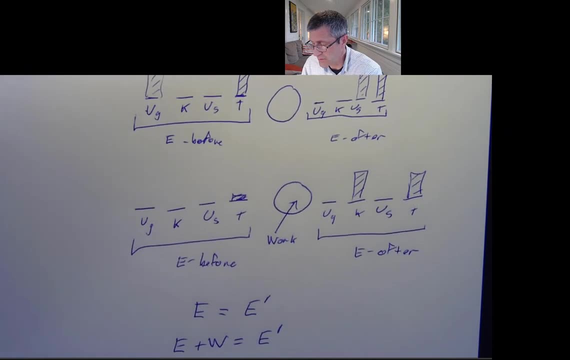 Right. So I can think about this as energy plus work is going to equal the energy afterwards. Now remember this. There it is. So remember the sign of work tells me something. So if I'm adding energy in, I'll have positive work. 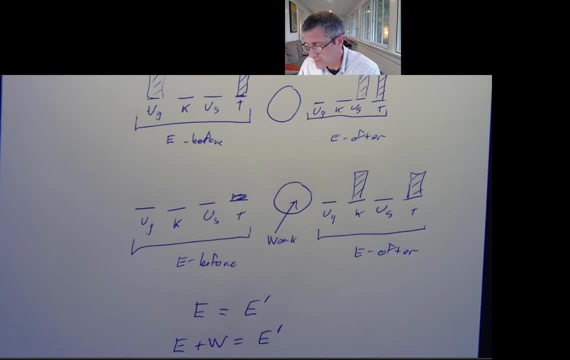 And if I'm taking energy out, I'll have negative work. So these two are the general forms of the equation. It says: well, here's my energy conservation: the absence of external forces. And here's my energy conservation with including external forces. 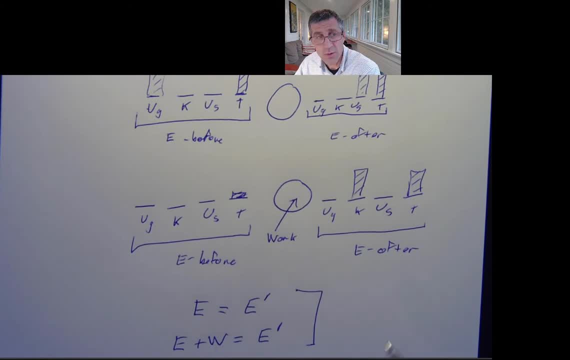 That can add or subtract energy from it. And now what I want to do is I want to get to an equation, right? So, for this first one, well, what am I doing? Well, I start with gravitational potential energy, right? 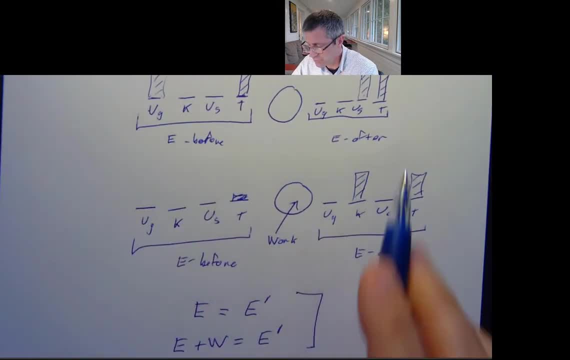 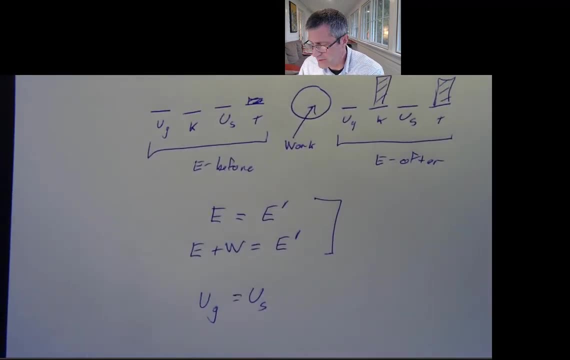 So that's all the energy I have before, And I end with spring energy, And now I can get to an equation from that if I needed to, And this is what we're going to be doing all the time. So we're going to start here, right? 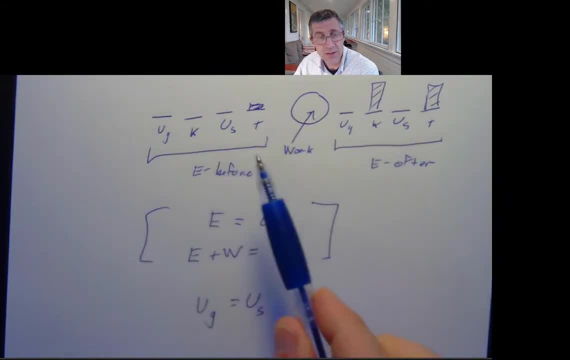 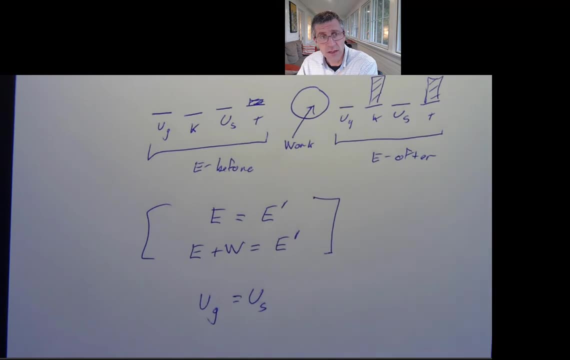 Start with one of these two equations And then take into account the things that are actually changing those. So we're going to see a number of these, These sort of diagrams, And this is the best in my mind. this is the best way to think about energy conservation. 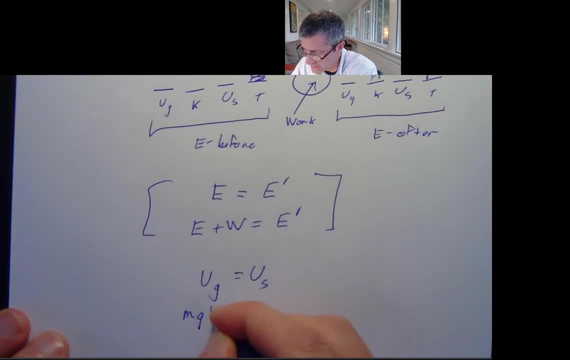 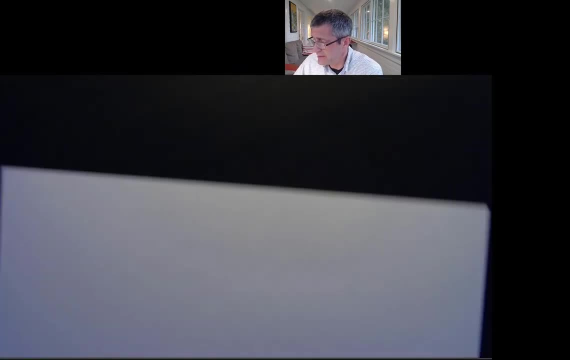 So we'll end up with a whole bunch, right? So this one is from close to the surface of the earth. One mgh is going to be one half kx squared, And then I can solve for whatever is missing. Let's think about in terms of like a roller coaster. 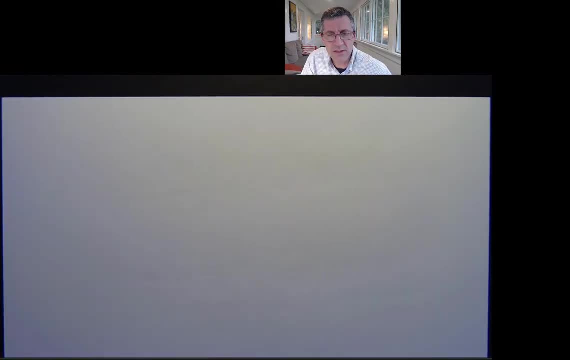 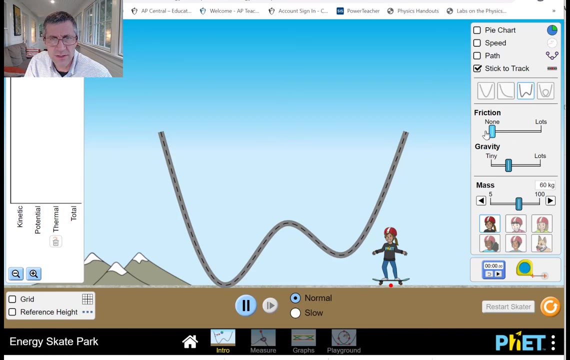 So let's go back to this energy skate park. Where is it? So? here it is. So this makes it more complex, right? So I'm going to go here, So I'm going to set friction to nothing Because I don't feel like worrying about it, right? 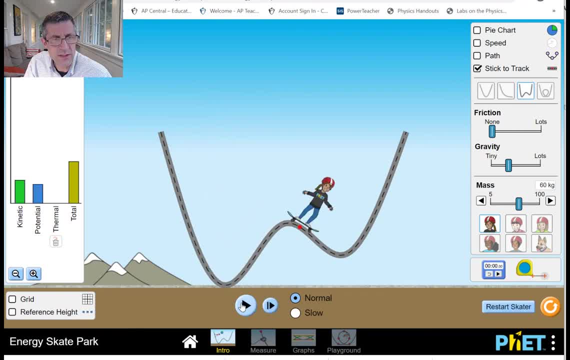 So she's going to go along And she's going to get to some point like here, right? So you've got a bunch of stuff going on. So she started with gravitational potential energy And it gets to this point. She's going to have some gravitational potential energy and some kinetic energy. 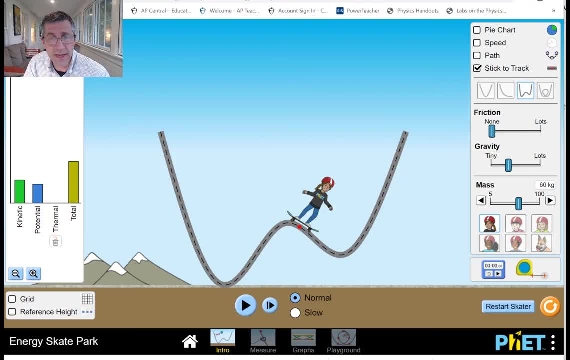 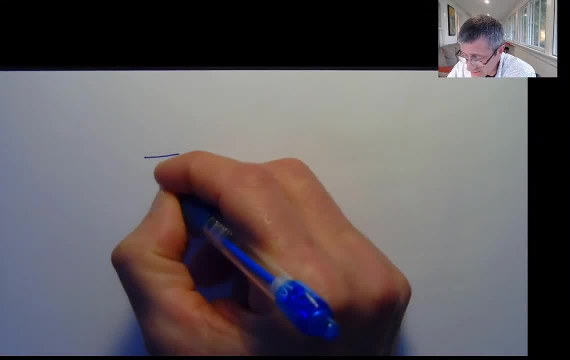 So let's take this into account, Let's draw this out using the energy diagrams And take into account the situation that she's in right now. So again, what am I going to start with? So I'm going to start with possibly. 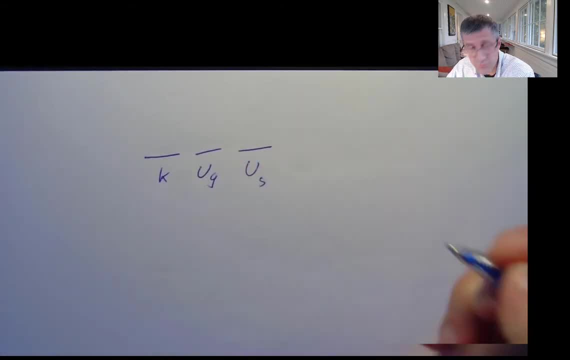 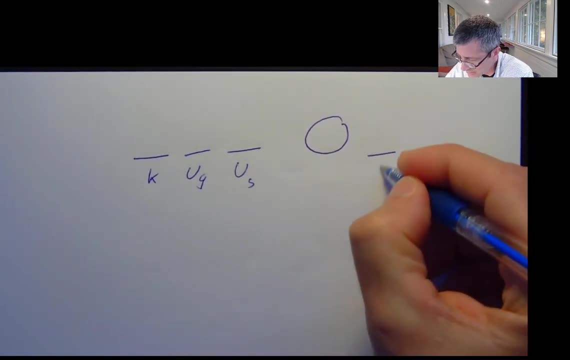 Kinetic energy, Possibly with gravitational potential energy, Possibly with spring energy, And then I can add or subtract, work, And then I'm going to end up possibly having kinetic energy, Possibly having gravitational potential energy, Possibly having spring energy. So in this case she started. 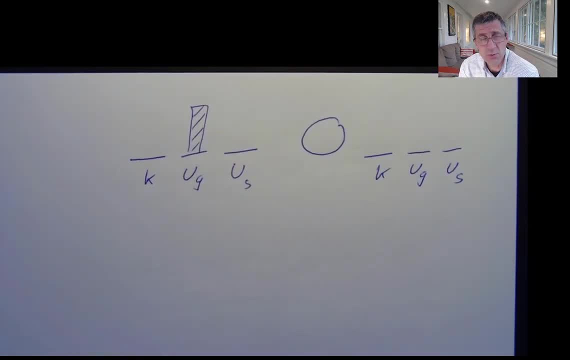 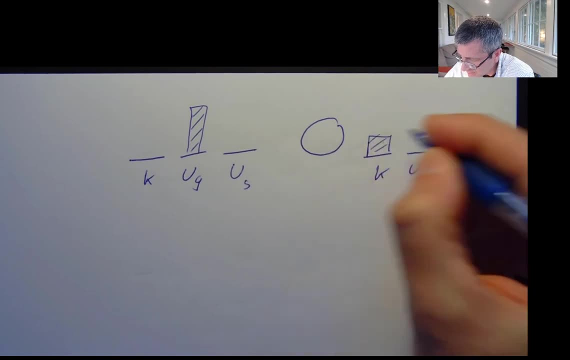 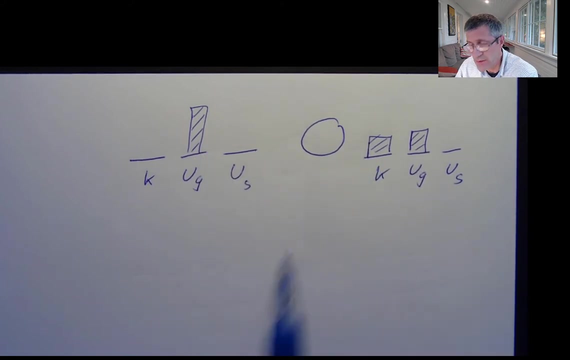 I set her up high, I did some work to get her going, But when she's going she's got gravitational potential energy. And then when she got to that point, she had some kinetic energy And some gravitational potential energy And these two bars are going to equal this. 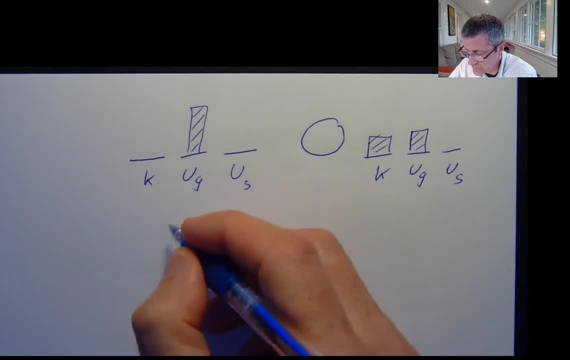 So there's no friction. I didn't add anything into or out of my system. So this is my energy before, This is my energy afterwards. I'm going to say my work is zero, So I didn't do any work on it. 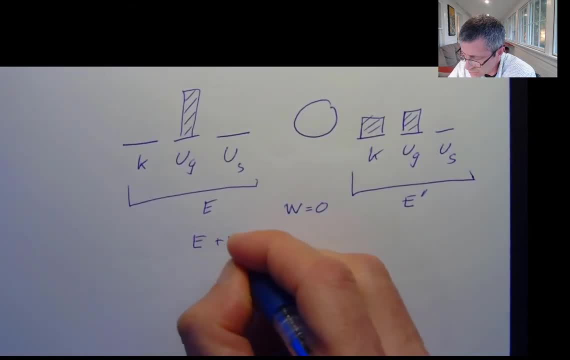 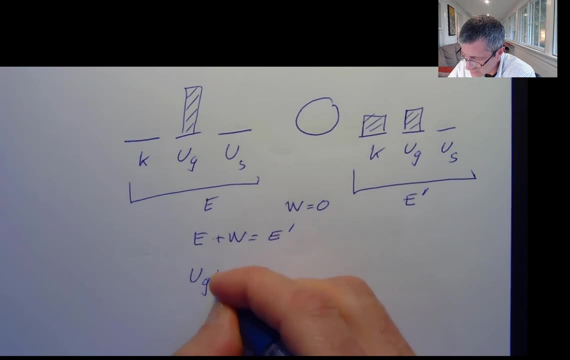 So now I'm going to write up my energy that I start with plus work. This is going to equal the energy that I ended with. This is zero, So I just started with, And this is going to be equal to K plus now my new gravitational potential energy. 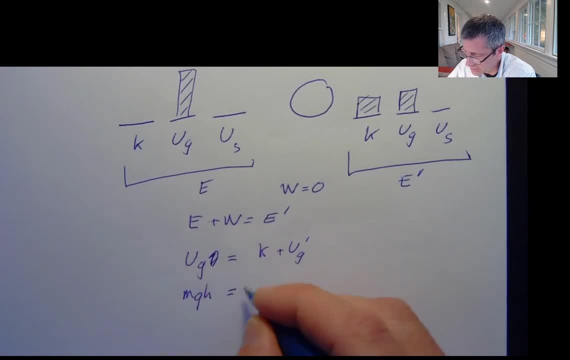 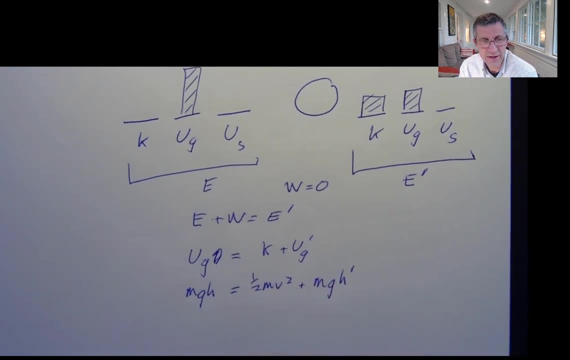 So I can say mgh that I start with is going to be equal to one half mv squared plus mg new h, And you may notice that in the absence of springs my mass is going to cancel, So it doesn't matter her mass. 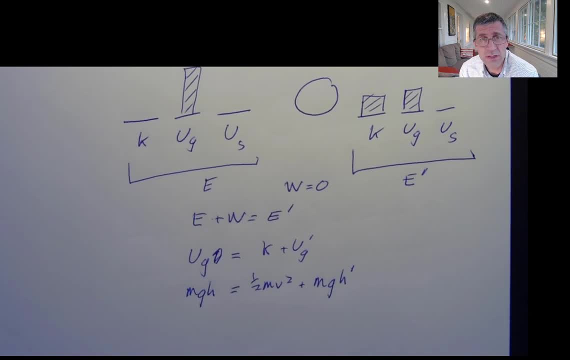 If we need to know velocity or her ending position or whatever it is, that mass is going to be irrelevant. So again, in energy, mass often cancels. As long as I don't have a spring, it's probably going to go away.